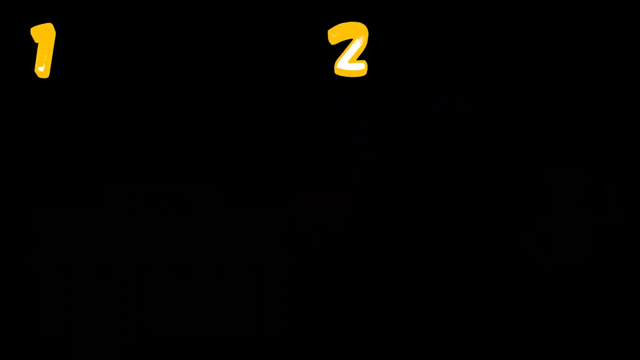 them to come back later. here the customer and you are faced with two options. the customer could either visit the store every day and check for the products availability- however, most of these strips would be pointless if the product is still unavailable- or you, as in the store owner, could. 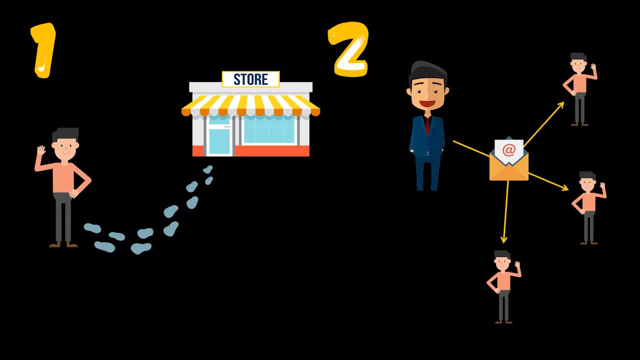 send an email to all your customers each time a new product becomes available. now, while this could save a few customers endless trips to the store, at the same time it could upset our other customers who aren't interested in these products, and they will most likely consider it spam. so what we need? 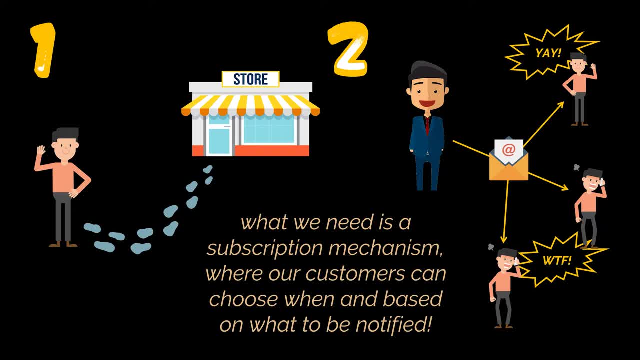 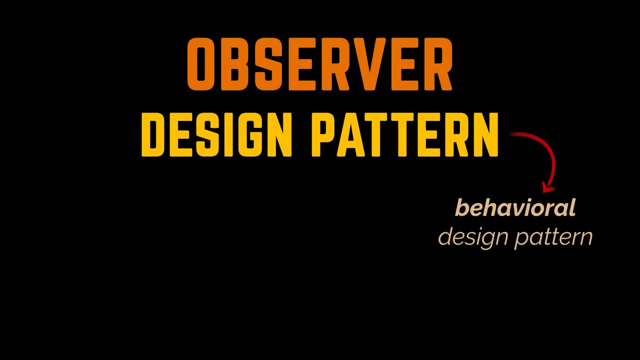 is kind of a subscription mechanism where our customers can choose when and based on what to be notified, or even if they want to be notified at all. and to design such a system there is no better way than to apply the observer pattern. the observer design pattern is a behavioral design pattern that notifies multiple objects. 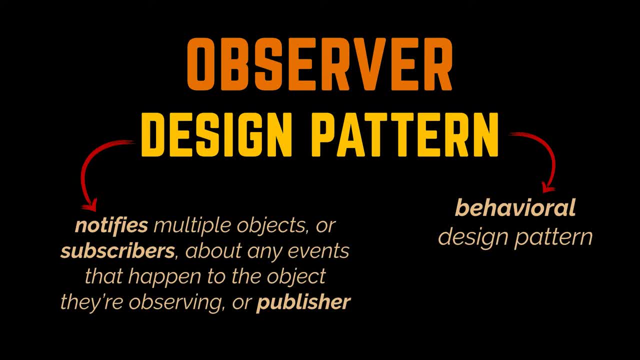 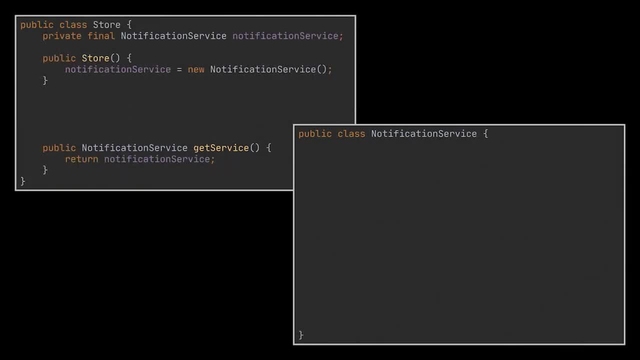 or subscribers about any events that happen to the object they're observing, or publisher. so, to implement our previous store customer scenario, we need to make sure that the customer is not completely isolated when también estamos en la casa del usuario. what we need is something like a notification service which will sit inside our store class. now this notification service should. 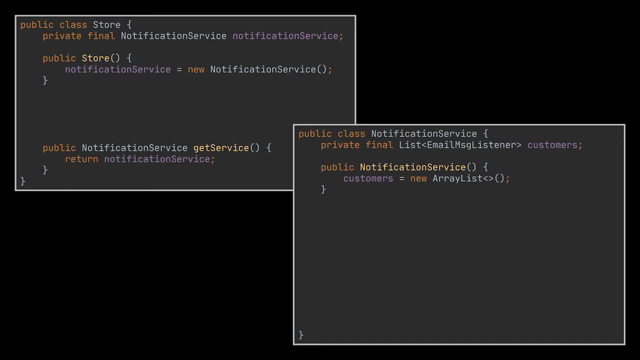 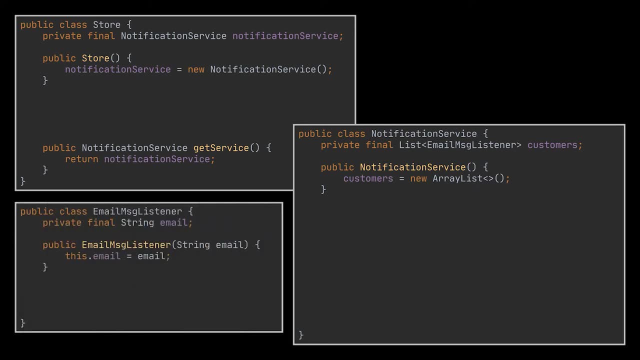 keep track of the customers or subscribers or listeners that want to receive our notifications via email. like we previously mentioned, these listeners will be represented by a list of email message listener objects, which will contain the email corresponding to each of our customer subscriber. this listener class will and should have an updated version of the customer€€. tämä. 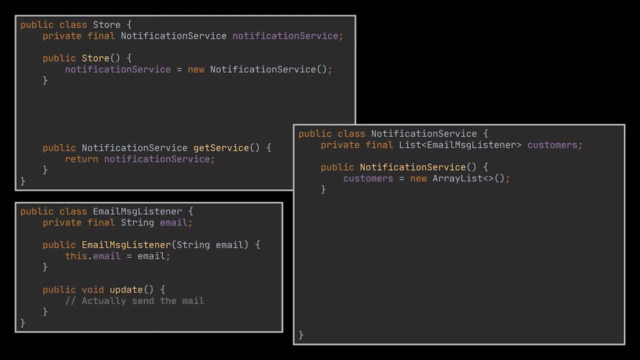 class-î adı. this listener class will and should have an updated version of our customer service, a link to that update method whose responsibility is to actually send the mail to the subscribed customer. Of course, and as previously mentioned, the service we are implementing should also grant. 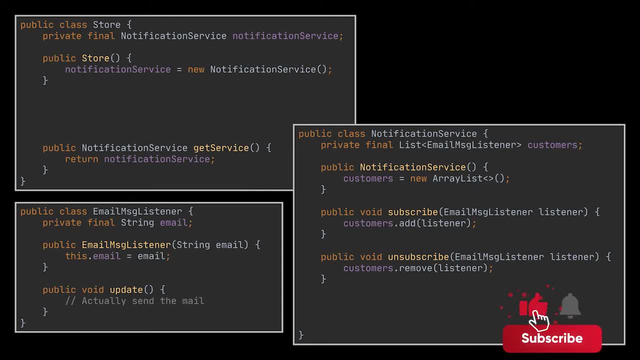 our customers the ability to subscribe and unsubscribe as they please from the notifications they are receiving. Now, when a new item arrives, we should have the ability to trigger this notification from our store class, and to do that, we added a new method in the store class. 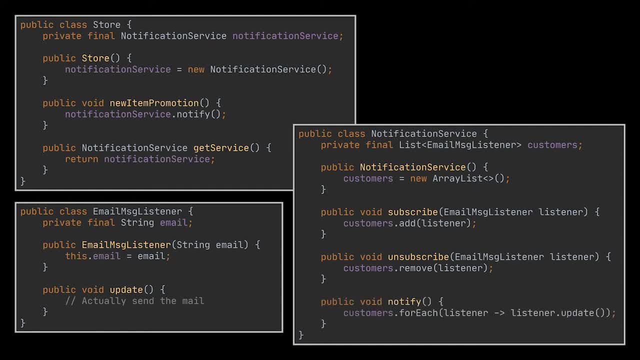 the new item promotion method. This method we'll call the notify method of our notification service, which will go over all our subscribers- or listeners in this case, and alert them via mail one by one, and that's it, Okay. I know some of you may be wondering why did we go through all this? 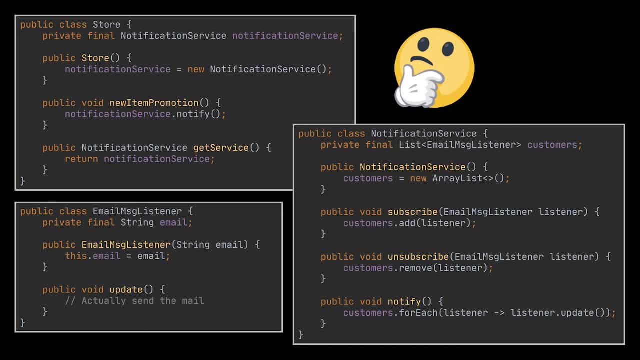 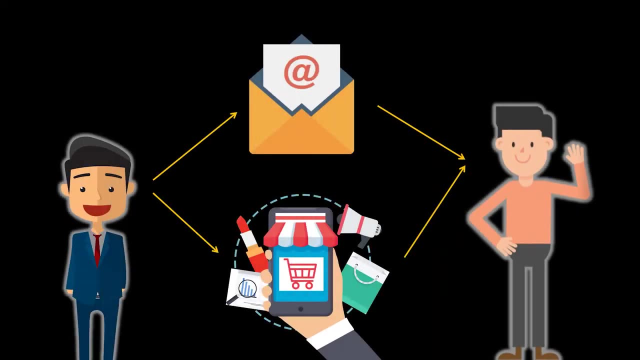 Why not just create a list, loop over it, send the emails and be done with it with a single method or class? Well, you see, while this may work, what we implemented is far more open for extension than what I just proposed. So suppose our store has a mobile application and now our customers? 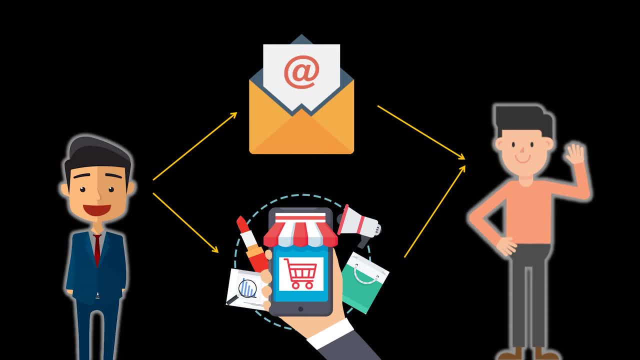 get to choose if they want to get alerted by mail or via a push notification on their mobile if their account is connected. If you had a single loop, that would be kind of hard to implement, but with the observer pattern it couldn't be easier. Take our current implementation. All we have to do is 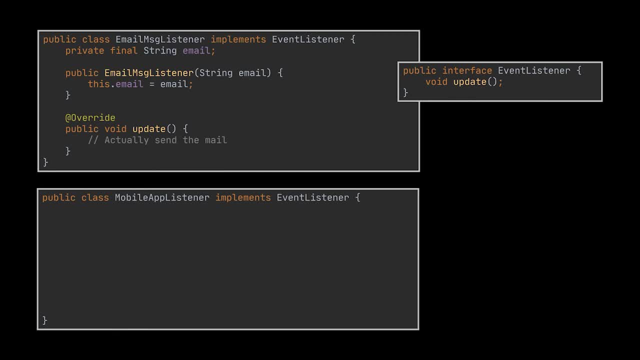 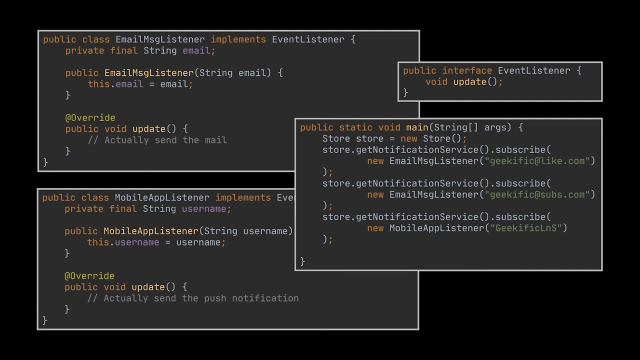 add another type of listeners and make both our listeners implement the same interface. This listener will work with usernames instead of emails, And its update method will send push notifications to these user accounts instead of emails. Now our client code will look something like this: We might have a store object along with 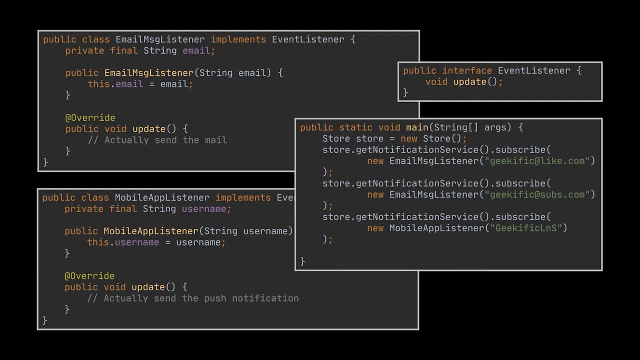 several subscribers, some via mail and others via push notification. When a new item arrives, all we have to do is call the new item promotion method and each subscriber will get notified via its chosen corresponding listener. Let's take this a step further and imagine we want to add: 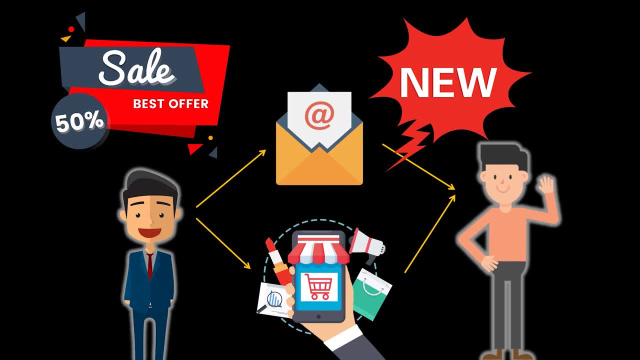 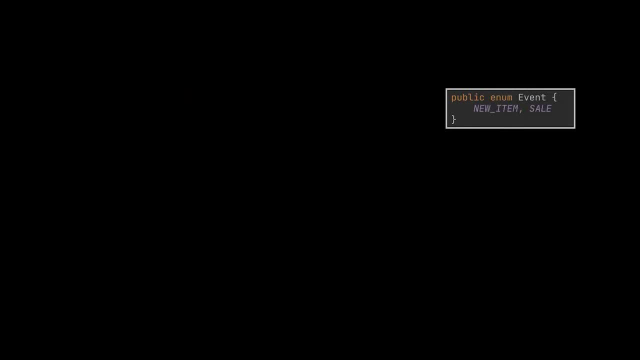 promotions or we want to notify our customers of the new item promotion method. Now we have to create an event enum and the values this enum can take are new item and sale. So we are going to give our customers the ability to subscribe to either new item events or sale events. The next 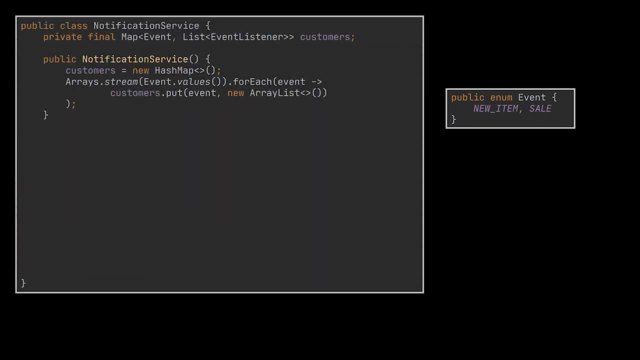 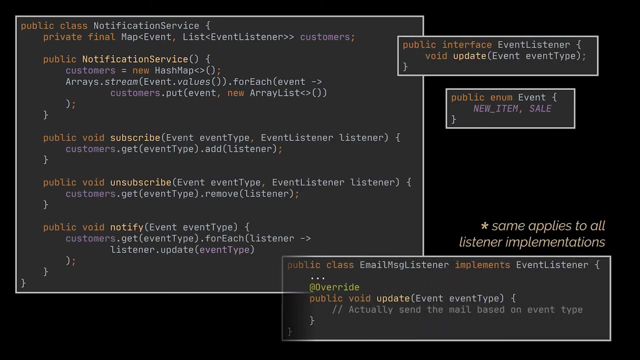 thing to do is transform the list of subscribers present in the notification service to a map. The key of this map will be an event, and the value of each key will be a list of the customers listening to that particular event. Finally, all we have to do is adapt the update. 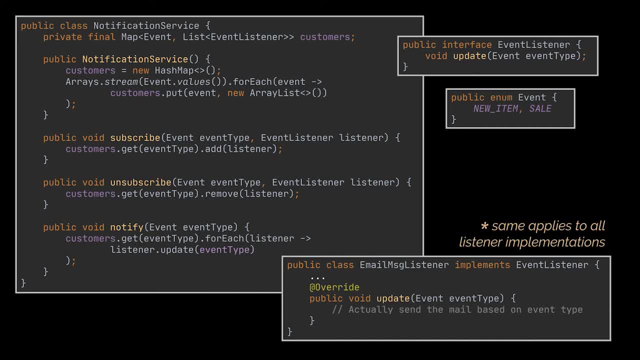 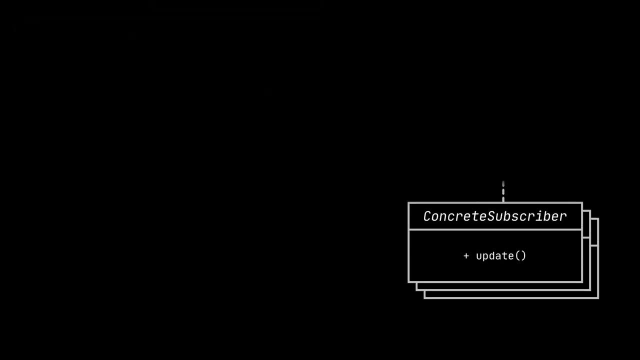 notify, subscribe and unsubscribe methods, to take into consideration the event at hand and consider that the changes we are doing should be applied on a particular list of listeners- the subscribers of a particular event- and not all of our subscribers. With the implementation now complete, let's go ahead and take a look at the structure, or